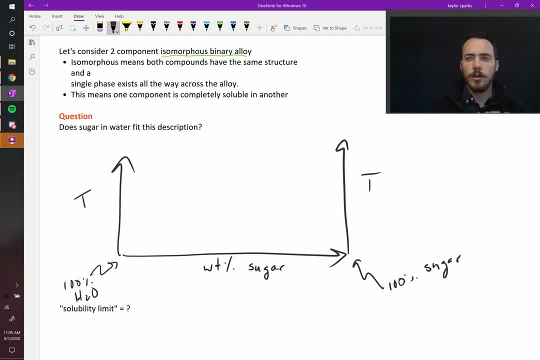 Still temperature. right, It's temperature on the y-axis, but you see that we're going from pure water all the way over to pure sugar. okay, So if we were to draw this figure, we would have to draw this figure. right, So we would have to draw this figure. 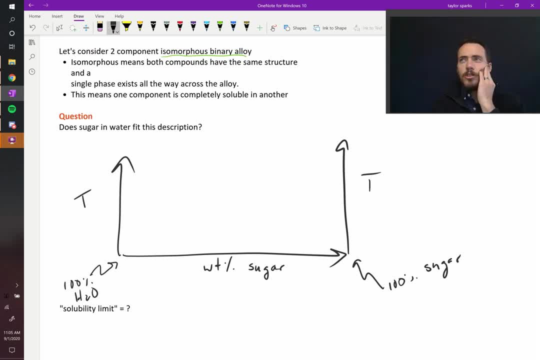 phase diagram. What do you know from your experience? Sugar and water: are they completely soluble, one with another? right, Because that's one aspect of an isomorphous binary alloy- is that they have to be completely soluble in one another. No, your gut feeling probably says. 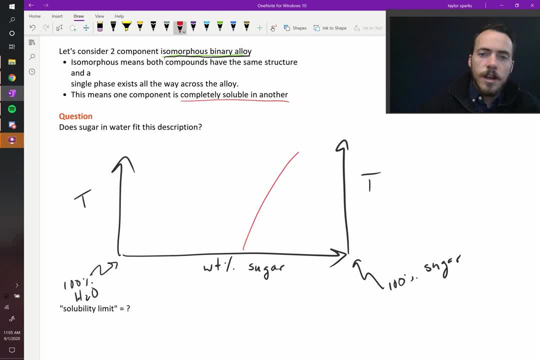 no, they're not completely soluble. There exists a line which is a function of temperature, and to the left of it we get what's called syrup, right. Sugar dissolved in water, okay, But if you're like my kid making Kool-Aid, he cannot resist adding way more sugar than can. 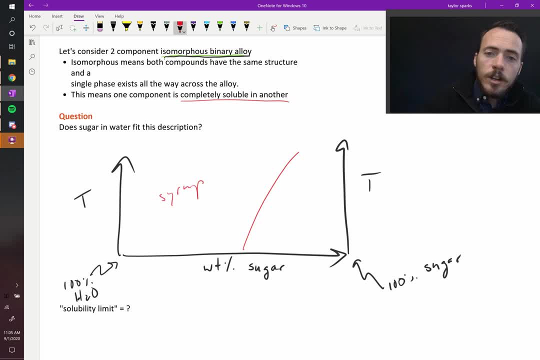 actually be dissolved into this Kool-Aid right, And so over here you end up with syrup plus sugar. So it's still syrup, like there's a certain amount of sugar that's dissolved in the water and there's a bunch of it that just isn't dissolved. if you cross over that line, 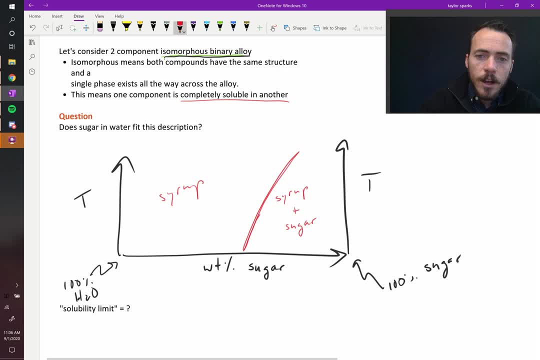 So this line- this is the key feature in this diagram here- It represents a boundary right And along that line you have an equilibrium between syrup and syrup and sugar. okay, And you know that if you do want to dissolve something, if you're trying to dissolve sugar in 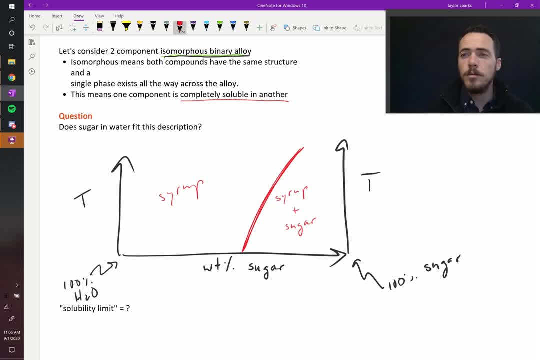 something that you should heat it up. Most times when you heat things up, the solubility increases, right, Instead of being able to host, let's say, this amount. if you heat it up to this temperature up here, all of a sudden, you can dissolve much more sugar into it, okay. 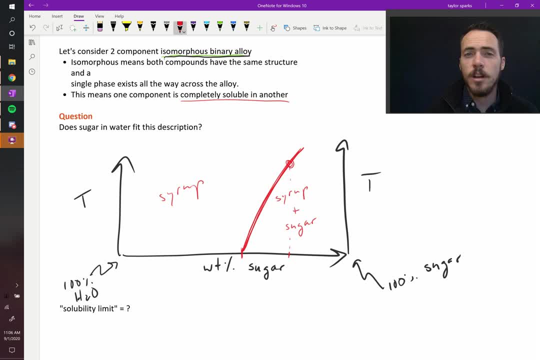 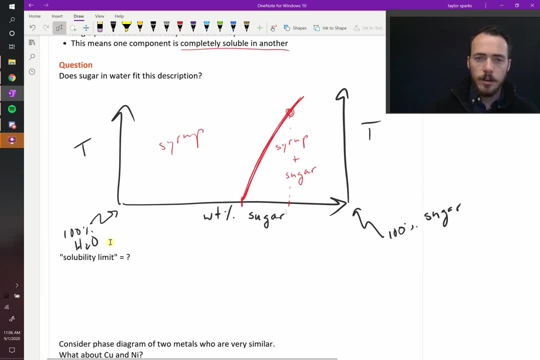 All right. So that is sugar and water. It does not fit. I just want to make sure that I'm describing the description of an isomorphic binary alloy, because it has this solubility limit right, which we've talked about. If you go to the 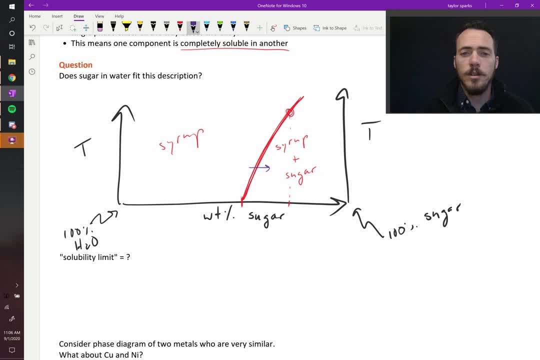 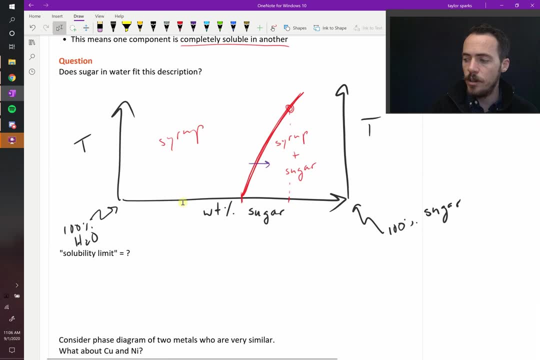 right of this line. you've passed the solubility limit. You cannot dissolve more sugar in this water. You start to precipitate out more sugar. It starts to become a separate, independent phase. Well, what about something like this? Consider the phase diagram of two metals that: 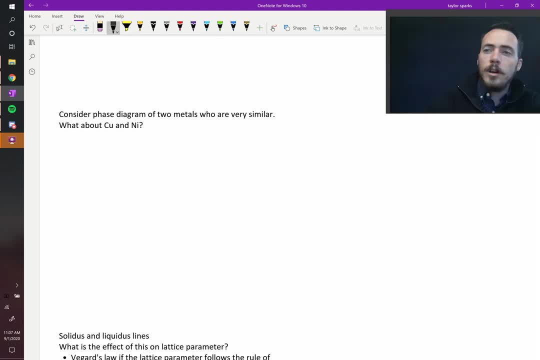 are very similar to one another. So do we have an example? Sure, How about copper and nickel? Copper and nickel. So I'm going to draw the phase diagram over here. When I'm doing copper and nickel, what happens to those two? Well, I'll do that with a one-to-one.